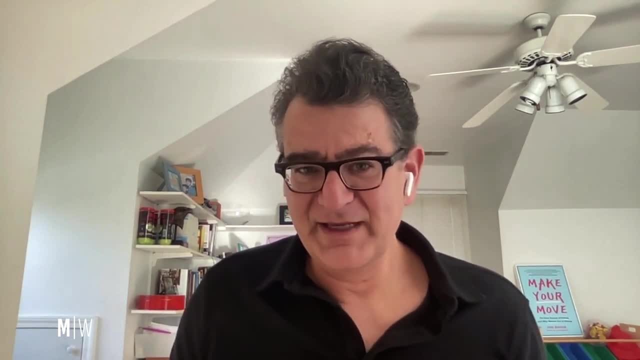 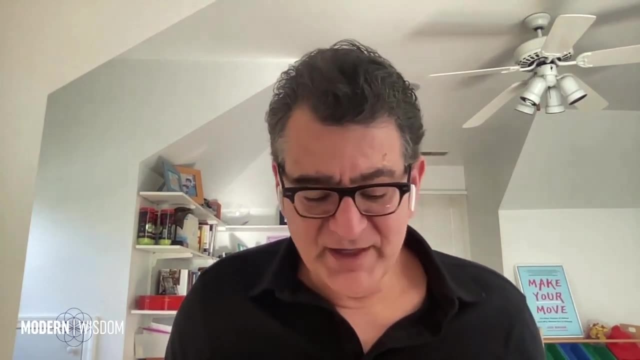 how differently kids talked about dating at various schools, depending upon the prevailing sex ratios, And I'll give you some examples here. So Rensselaer Polytechnic Institute, which is kind of a science and engineering school in upstate New York, RPI- RPI is about 70% men, 30% women. 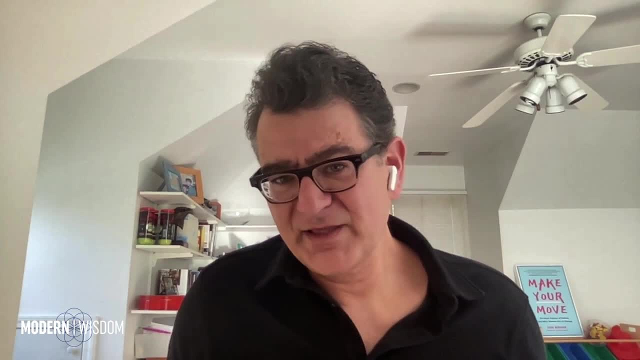 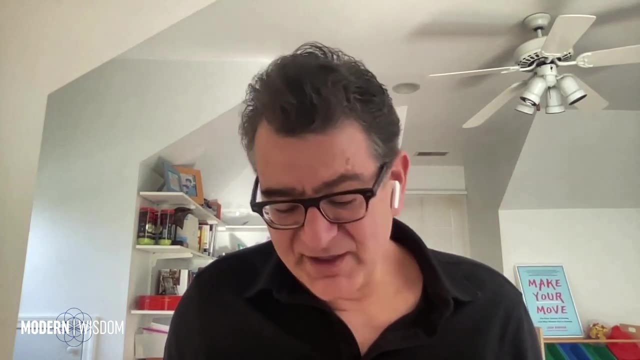 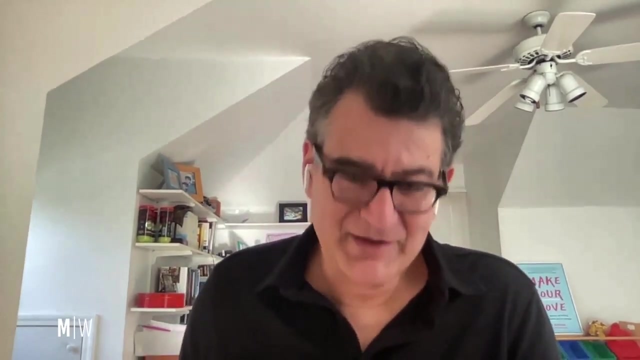 to you know, more than two men for every one woman. And here's what students said about dating at RPI. More people are involved in relationships. girls seem to become stuck up because they're in choosy Caltech, which is, you know, California Institute of Technology in California. And if you 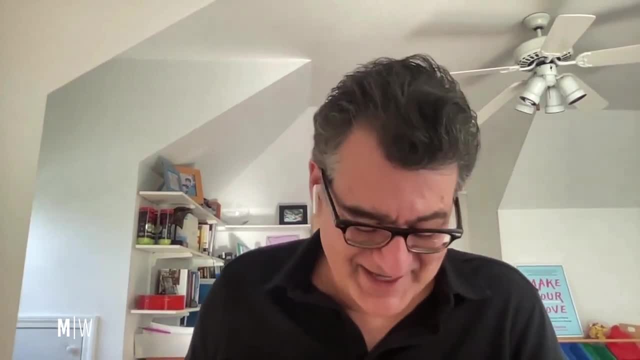 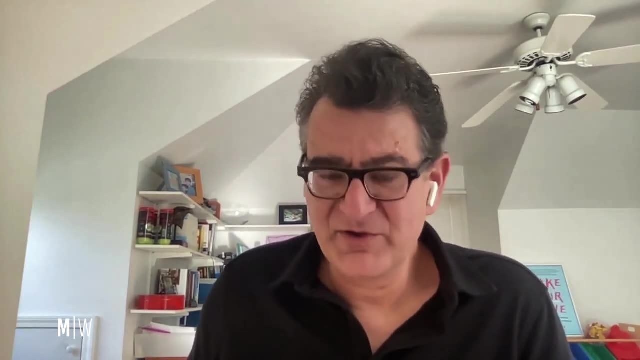 remind me. I have an. I have a funny story about Caltech, which I can add at the end. Caltech is 60-40, 60% men, 40% women. three women for every two, three men for every two women. Here's what. 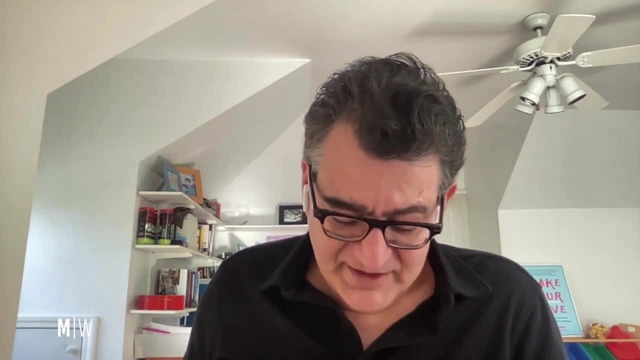 students said there about dating. Students here tend not to date but have relationships. breakups are rare and many couples get married after dating, So it's really important to know what they're dating. So if you're dating a woman, you're dating a man, you're dating a woman. 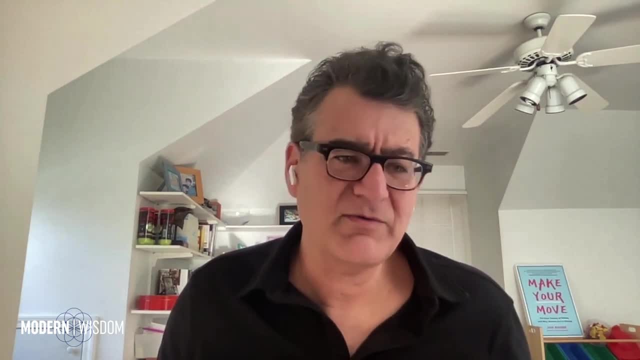 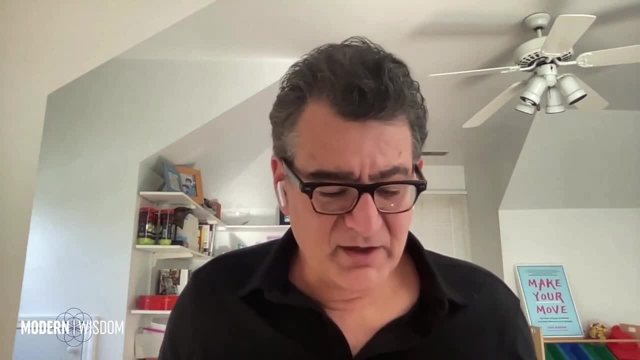 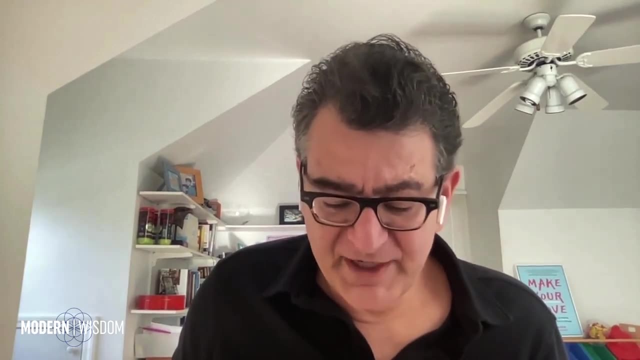 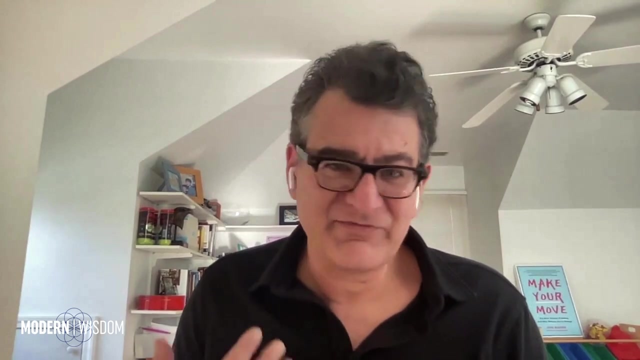 guy when it came to like what I remember about college. So Tufts University, which is in suburban Boston. Tufts is 50-50.. Halfway through sophomore year people begin to pair off and generally stay paired off through junior and senior year. That's familiar to me. That's what I 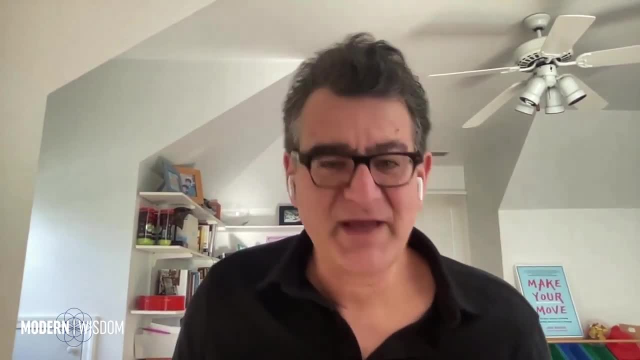 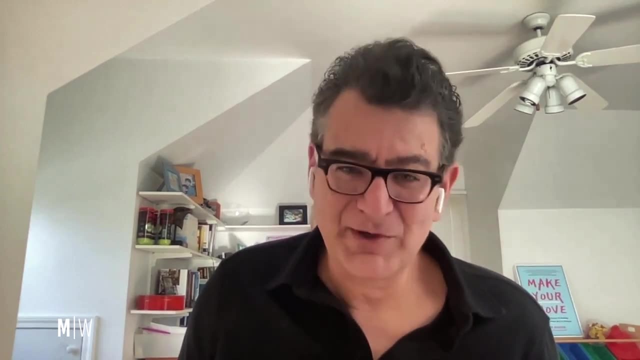 remember, University of California, which is a university in the United States, is 50-50.. University of Miami, which has a reputation as a big party school, but it also happens to be 50-50.. And here's what students say about dating there. Random hookups are common in the beginning. 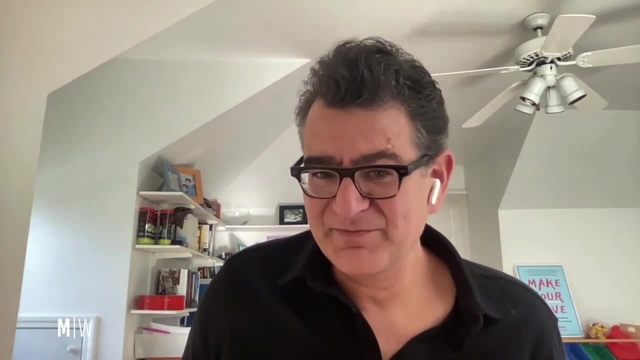 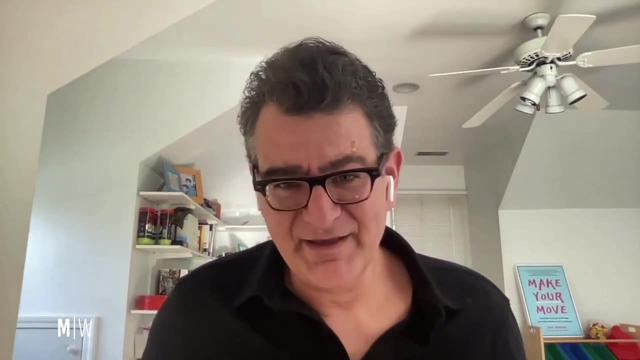 but after a few months or a year, relationships take over. So compare that- the schools that are either more men than women or 50-50, to some of the schools that are disproportionately female. I'll start with New York University in New York City. 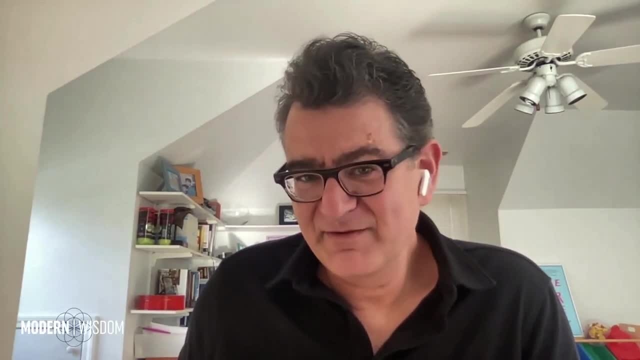 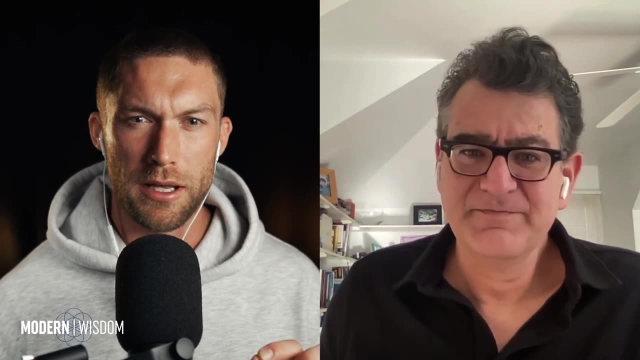 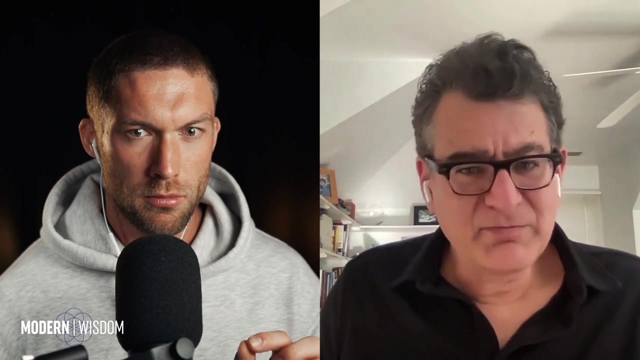 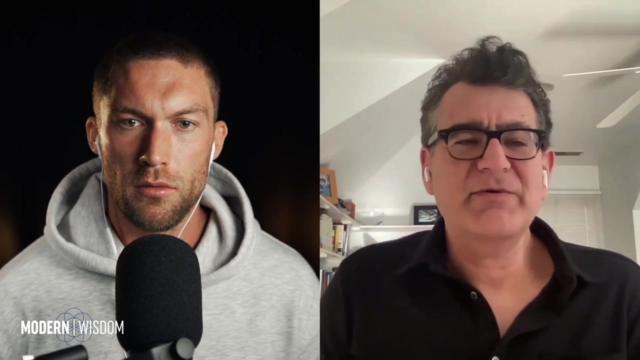 NYU is 61% female, 39% male. Is that that's about representative, typically, I think, on average for most colleges. now, It wasn't when I wrote them, It was more like 75-35.. It was more like- I'm sorry, it was closer to 58-30-42. 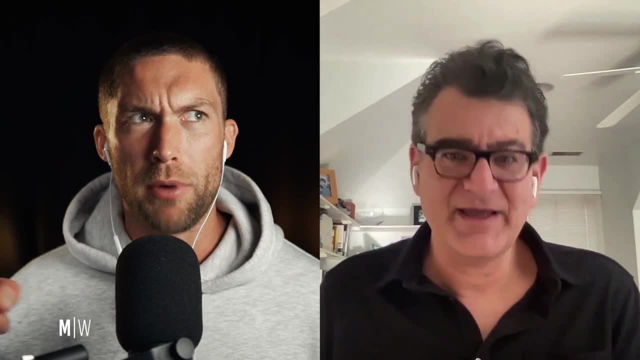 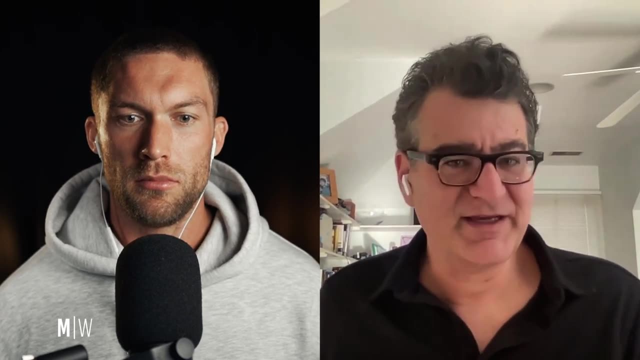 42,. yeah, I mean, I wrote them, But we're now looking by 2030, we're going to be, But now it's, yep, I think, this year's graduating class. I think you're right, I think at least in. 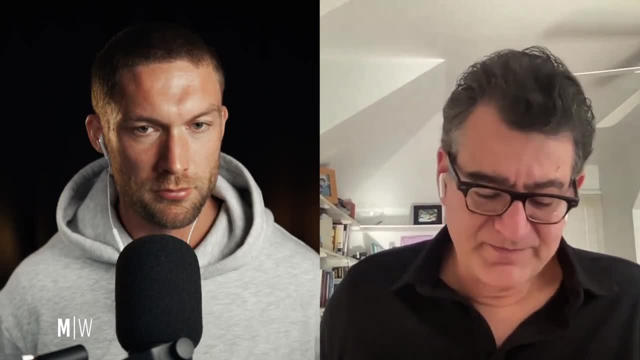 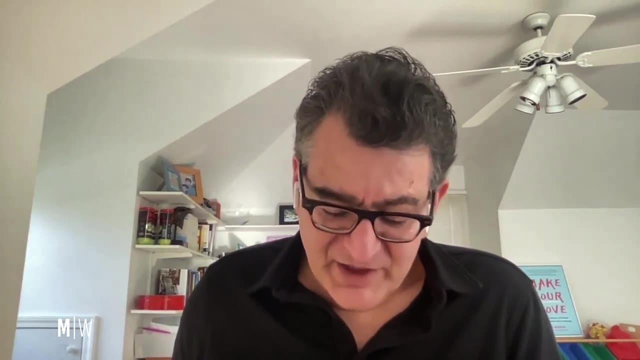 the US it's 60-40.. It's going to be bang on. So NYU, New York University. here's what kids say about dating. at NYU, Guys take advantage of the male-to-female ratio and most have no plans of settling. 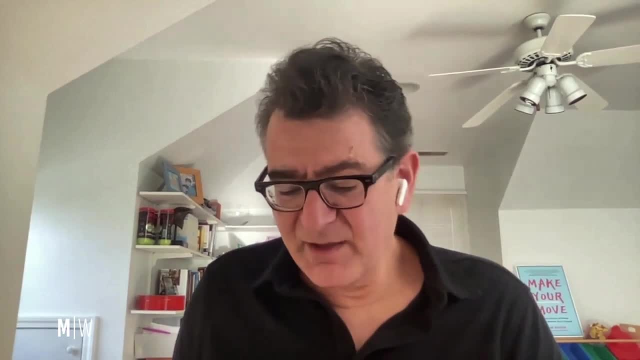 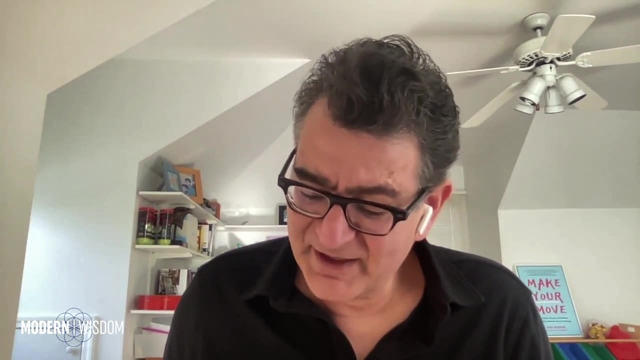 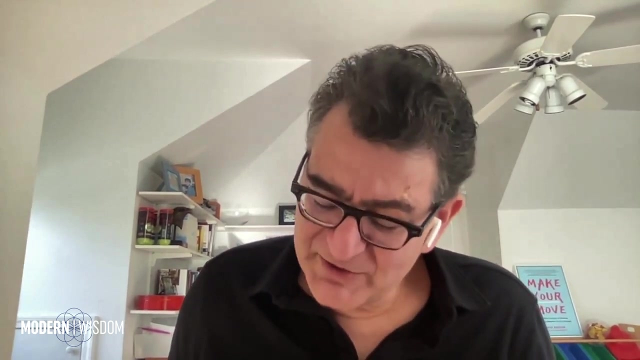 into a long-term relationship. Boston University, where actually my, My son is a senior BU is 62% female, 38% male. Here's the comment. Freshman year is a sexual explosion. There are girls to go around and around again. 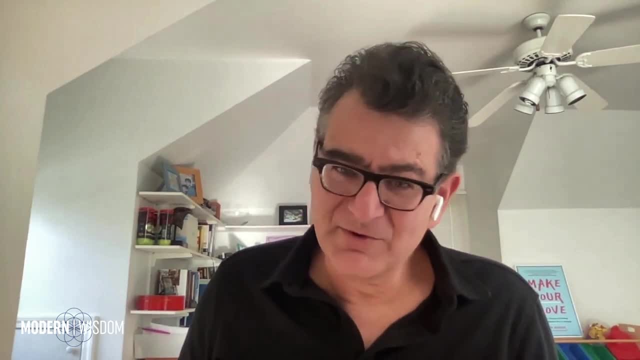 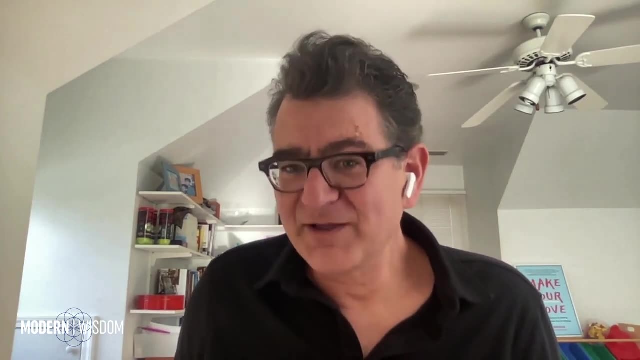 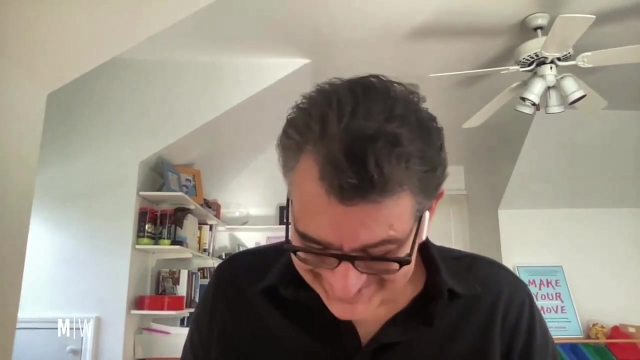 And lastly, Sarah Lawrence College, which used to be an all-girls school in suburban New York. It's now co-ed, but it's 75% female, 25% male, three women for every one man. You could probably guess what I'm about to read to you, but let me share. Quote: the girls complain about loneliness, the guys get more than they can handle and mindless one-night stands are rampant. So for me, doing the college research really kind of showed how these prevailing sex ratios don't just affect the statistical odds of getting into a relationship, but they change. 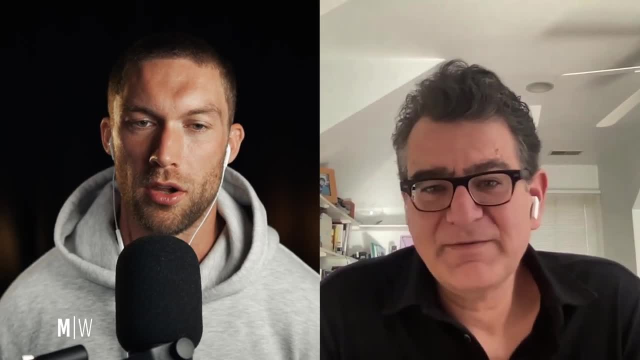 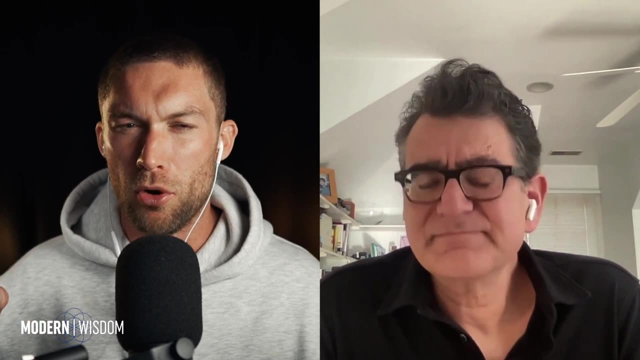 culture, they change behavior as well. Yeah, and rolling the clock forward, The people that graduate from those colleges. presuming that men and women drop out at similar rates, I think men might drop out a little bit more than women actually, but probably. 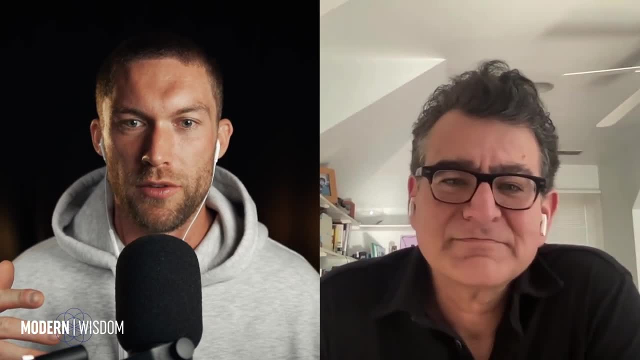 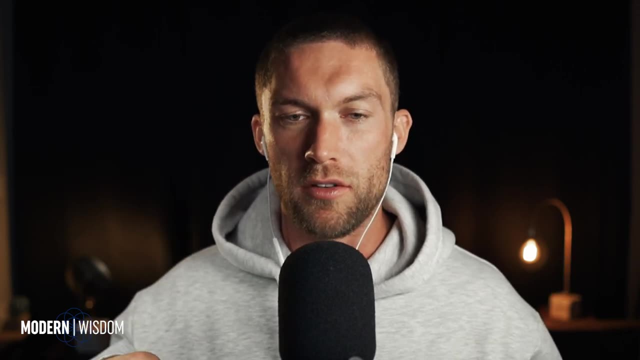 not enough to rebalance this sex ratio that we've got And I think that, yeah, you'd be about right at saying 60-40 women to men, but by 2030, the projection is two-thirds women to one-third men at a four-year US college.